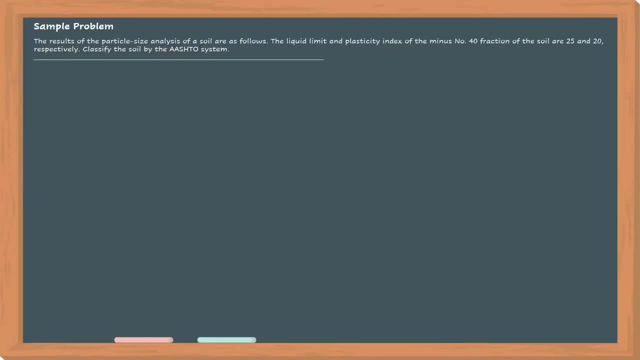 The results of the particle size analysis of a soil are as follows. The liquid limit and plasticity index of the minus number 40 fraction of the soil are 25 and 20 respectively. Classify it by the AASHTO system. So this is the particle size analysis result. 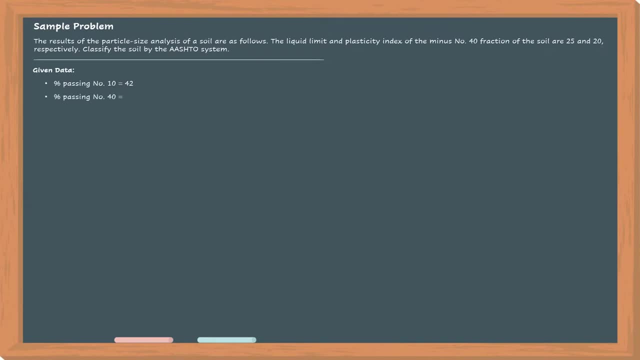 Passing number 10 is equal to 42.. Passing number 40 is equal to 35.. Passing number 200 is equal to 20.. So the liquid limit and the plasticity index are given. So before going to the solution, it would be best if we have a copy of the AASHTO classification table. 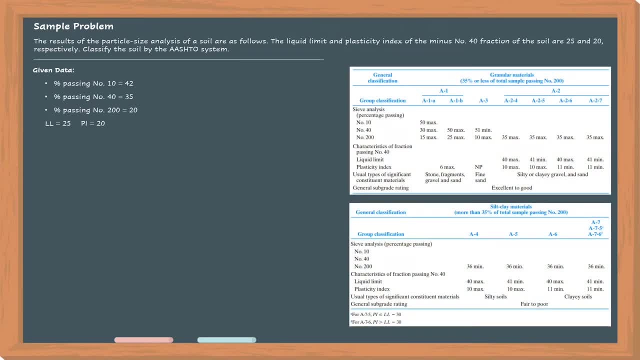 Just like shown here. So you can download this one through the internet Or you can print a copy From the geotechnical engineering book of Braha Das. Okay, so let's start the solution Number 1.. Since only 20% of the soil passes number 200, the soil is considered as granular. 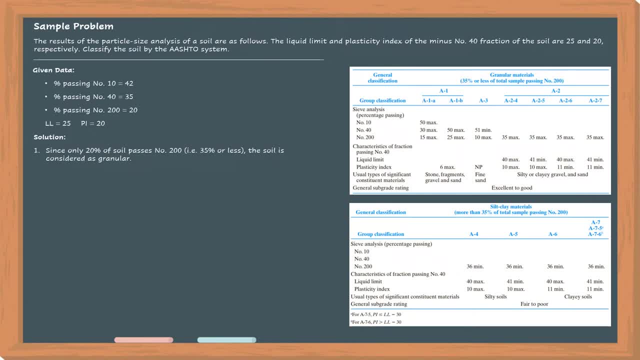 So the boundary point of granular and sealed clay material is 35%. So that means, just like in this table, if the percent passing number 200 is equal to 35% or less, it is considered granular. If more than 35%, so it means 36% and above, it is considered as sealed clay materials. 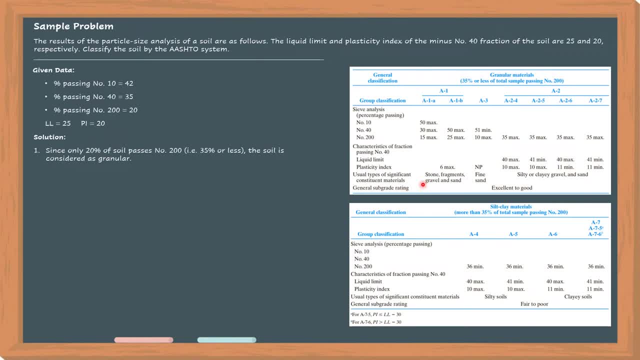 So we can therefore initially conclude that it can either be A1, A3, or A2.. Okay, Next, The soil is probably not A1 and A3. Why? Because the characteristics of fraction passing number 40 will not satisfy their criteria. 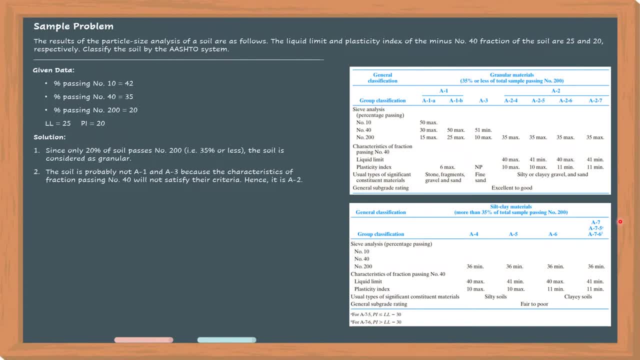 Hence it is A2.. So what is the characteristic pass of fraction, passing number 40?? So for A1, for it to be classified as A1, the liquid limit. it should not have a liquid limit Because it's non-plastic. 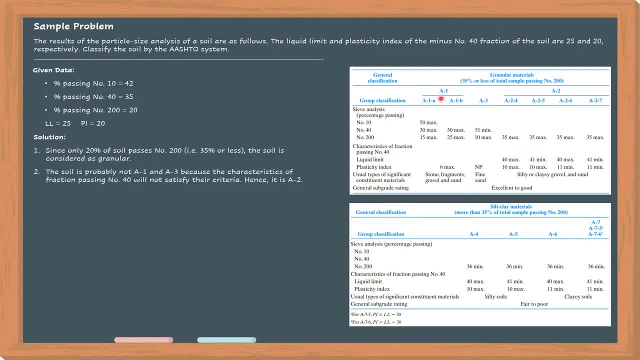 Um Plastic, There is an amount of silt material, but it is not enough to determine the liquid limit. So the plasticity index is the only criteria for A1. And the maximum value is 6.. But the given plasticity index of the soil is 20.. 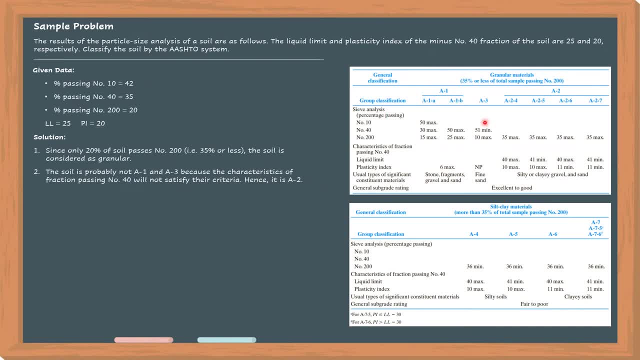 So crash out of A1.. And then for A3, it's non-plastic, So it doesn't have plasticity index and liquid limit, But it is not probably A1 or A3. So let's go to A2.. It can either be A2, A2-4, A2-5,, A2-6, or A2-7.. 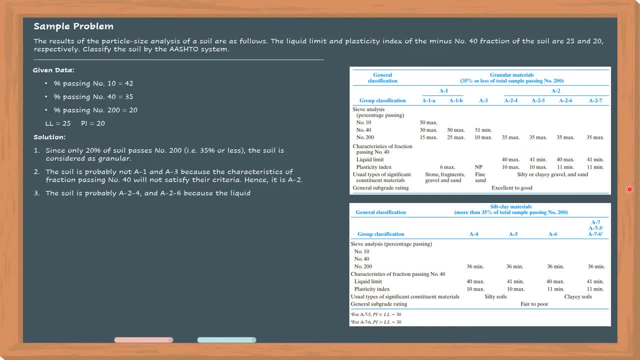 Next, the soil is probably A2-4 and A2-6 because the liquid limit is below 40. So for it to be classified as A2-4, the liquid limit must not exceed 40. Because it is 40 max. 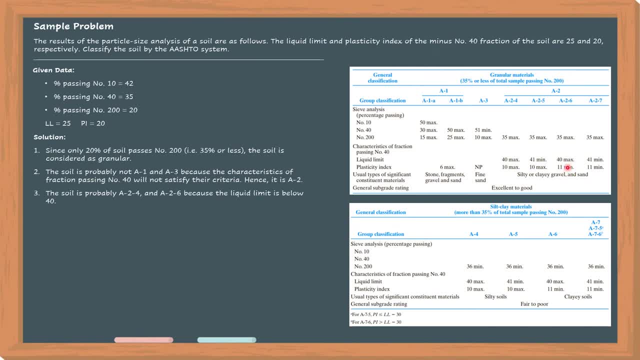 And for it to be classified as A2-6,, 40 is its liquid limit. So we will now look at the plasticity index. So, since the plasticity index is equal to 20, So where should the 2 satisfy the criteria? 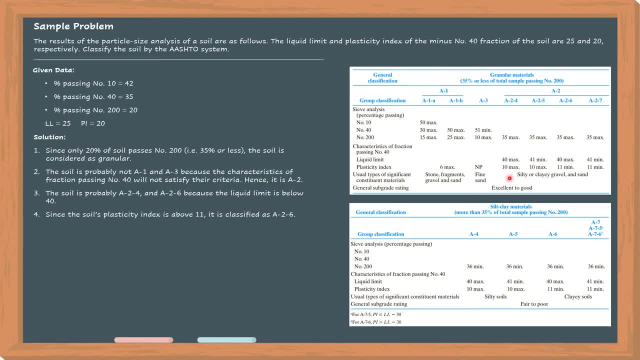 Probably A2-4, because the plasticity index limit is 10.. And then for A2-6.. A2-6.. A2-6. Its minimum is 11.. So therefore we can say that the soil's classification is A2-6. 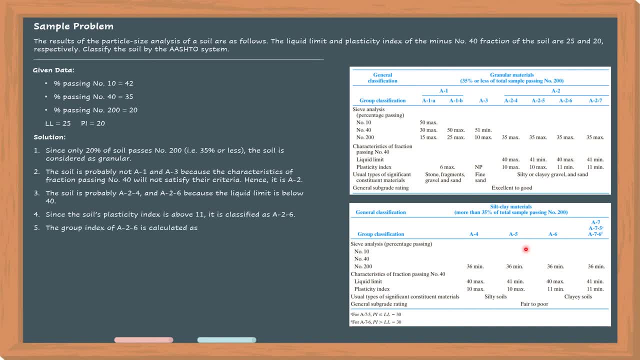 And then, after determining the classification, we now compute the group index. So the group index is computed as: 0.01 times F-15 times Pi-10. Where, Where F is the percentage of the fraction passing number 200. So F is equal to 20..